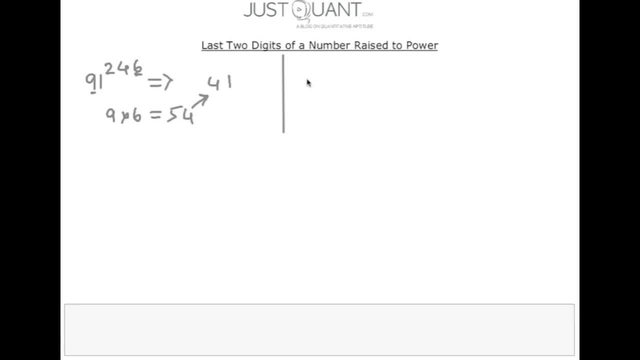 example. I have an example, say 341.. Since 341 ends in 1,, 341 to the power of 122 also will end in 1.. And the 10th digit is obtained by multiplying the 10th digit in 341,, that is 4, with the units digit in. 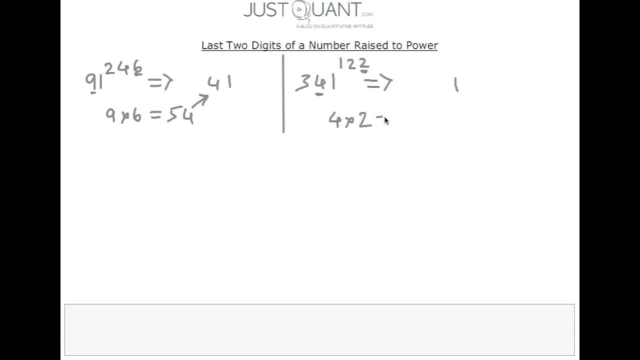 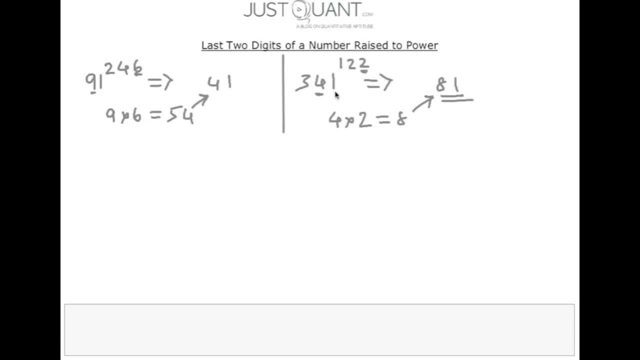 this is the 10th digit. So this is the 10th digit. Hence the last two digits of 341 to the power of 122 are 8 and 1.. In general, if you have a number which is in the form x to the power of y, where x is: 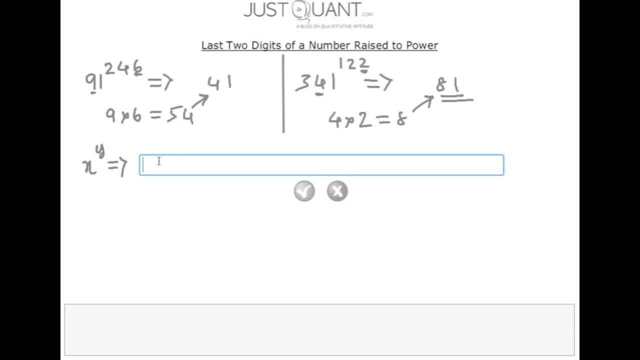 a non zero integer and y is a positive integer, Then if x ends in 1, x raise to y is equal to 0. So this is the 10th digit. So this is the 10th digit. So this is the 10th digit. So. 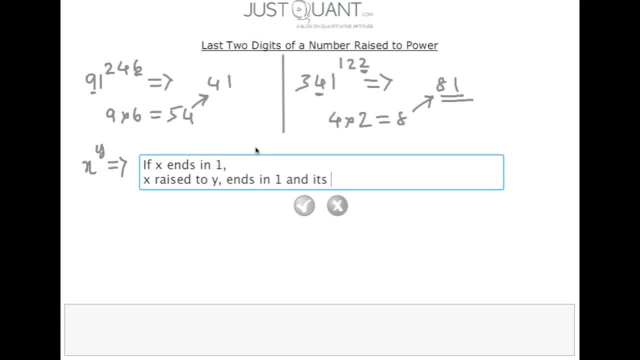 ends in 1 and its 10th digit is obtained by multiplying the 10th digit in the base, that is, in x, with the units digit in y. So this is the case when your number or the value of x ends in 1.. What if the units digit is other than 1?? So, based on the value of the 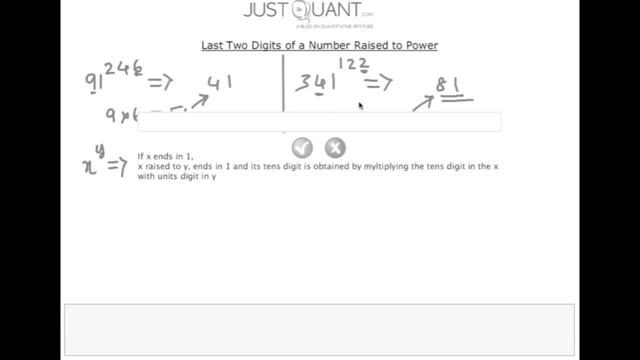 units digit. we categorize the solution into 4 different cases. Case 1 is when the units digit in x is 1.. Case 2 is when the units digit in x is either 3 or 7 or 9.. And case 3 is when the units digit in x is. 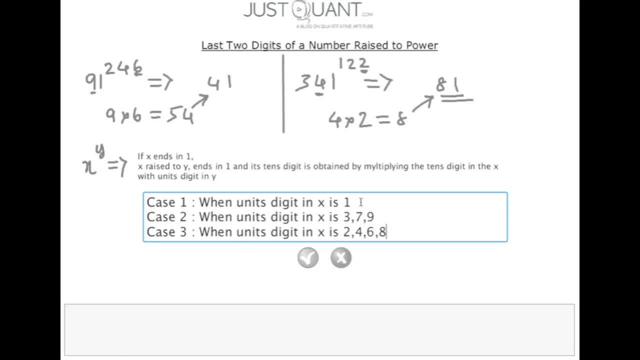 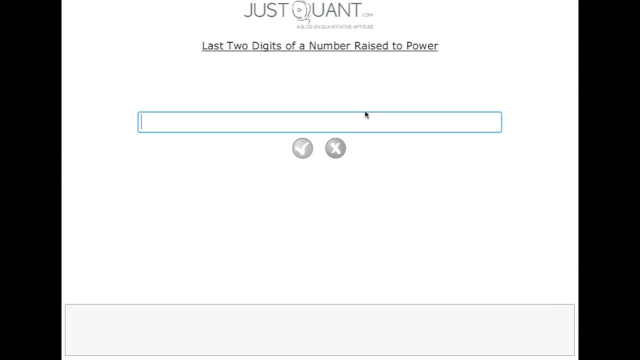 either 2 or 4 or 6 or 8. and case 4 is when the units digit in x is 5. we have just seen the first case. let's have a look at the other cases in detail. okay, let's look at case 2, where the units digit is either 3 or 7 or 9. let's again 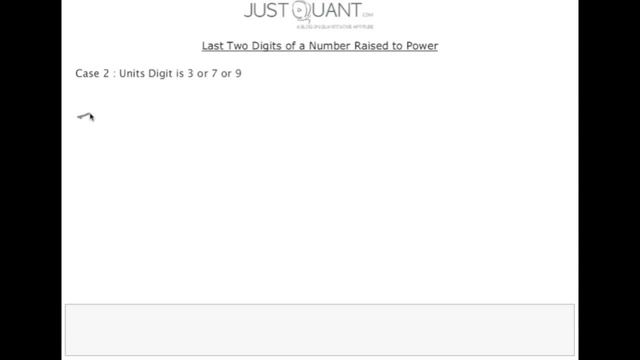 consider an example: says 79 whole to the power of 142. here we see that the base ends in 9. one of the easier ways of solving this is by converting the base into a number that ends in 1. we know that 9 square ends in 1, so 79 square will also end in. 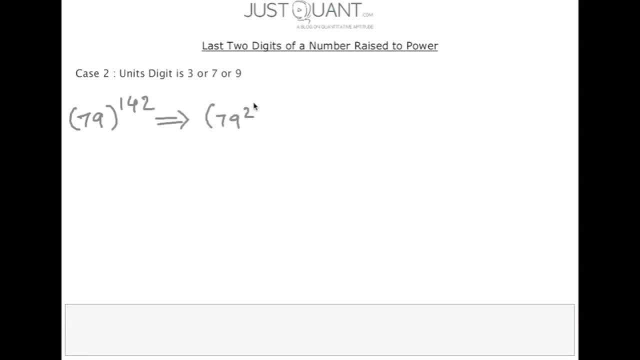 1. hence I write this as 79 square whole to the power of 71. now, since we are interested in the last two digits of a number, the last two digits of 79 square are 4 and 1, so 41 whole to the power of 71 is what we get now. this is similar to our case 1. 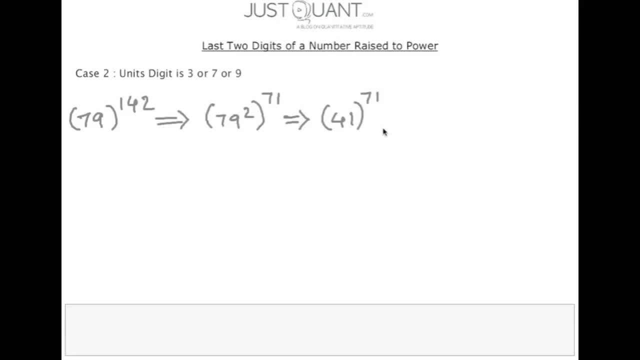 wherein the unit digit is 1. hence the last two digits will be 1 and the 10th digit is optimal, multiplying 4 with 1, which gives me 41. hence the last two digits of 79 whole to the power of 142 is 41. 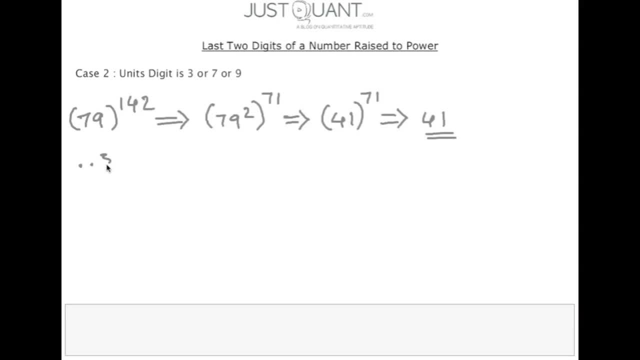 now, what if your base ends in 3? okay, here x is positive integer, dot dot represents the digits previous to 3. okay here, we know that 3 to the power of 4 ends in one. so the 4th power of a, a number whose units rigid is 3, will also end in 1.. Hence I will write this as 3 to 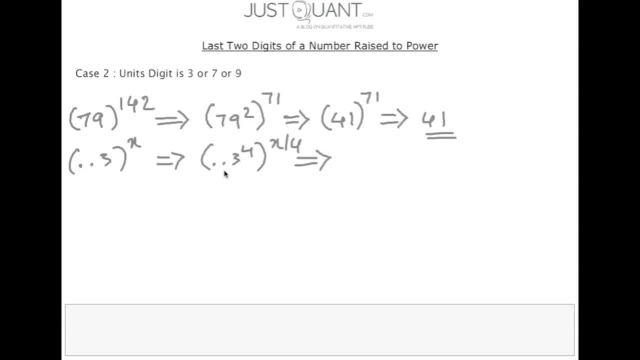 the power of 4 whole to the power of x by 4.. So this will end in 1 whole to the power of x by 4.. This again is similar to case 1.. Hence I can get my last two digits using: 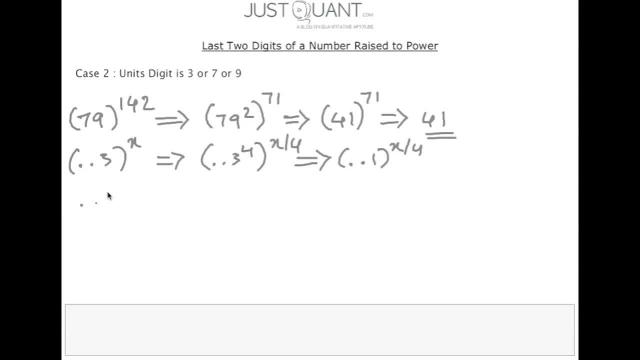 the technique involved in case 1.. Similarly, for digit that ends in 7, I can write this as whole: to the power of x, 7, to the power of 4 ends in 1.. Hence power of x by 4, which. 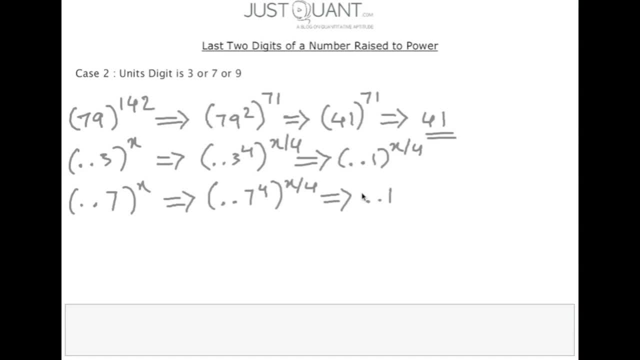 gives me 1 whole to the power of x by 4.. In general, what we do is, whenever we have a number in the form of x to the power of y, Then x ends in either 3 or 7 or 9. Then we convert our x- that is our base- into a number. 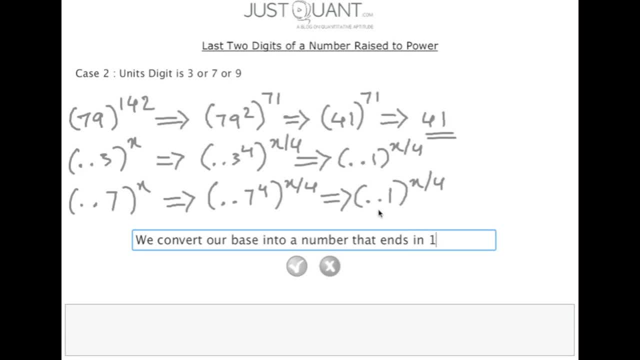 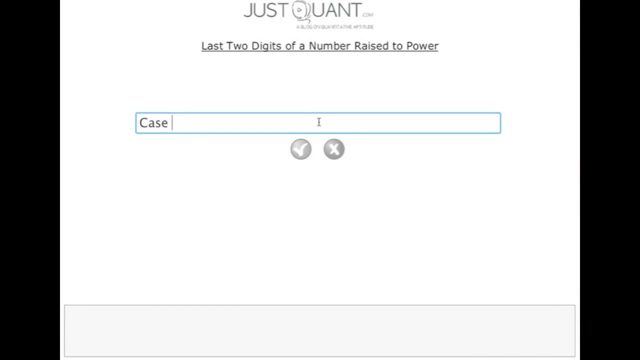 that ends in 1 and then apply case 1.. Now let us look at the next case case, where the units digit is either 2 or 4 or 6 or 8.. Our next case, case 3, units digit is either 2 or 4 or 6 or 8.. Before we solve problems on this case, the 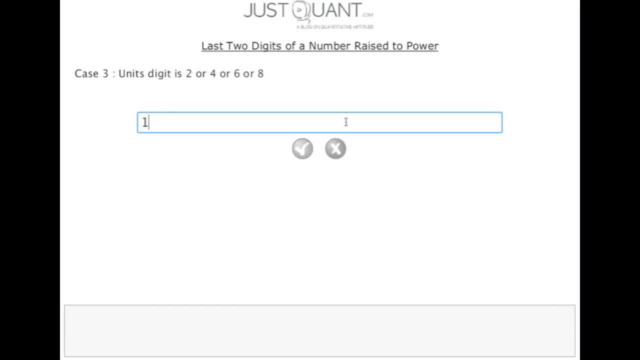 certain points that we are supposed to remember. that is 2 to the power of. that is 2 raised to 10 ends in 24, and 24 raised to an even number, ends in 76, and 24, raised to an odd number, ends in 24, and 76, raised to any number, ends in 76.. 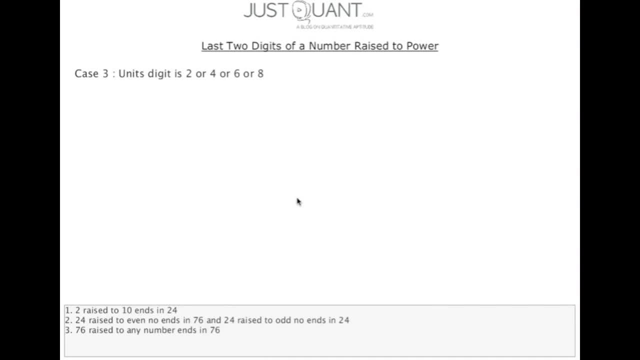 So, keeping these points in mind, let's try to solve some simple problems based on this particular case. Let's start with calculating the last two digits of 2 to the power of 1056.. I can write this as 2 to the power of 10, over to the power of 105, into 2 to the power of 6.. 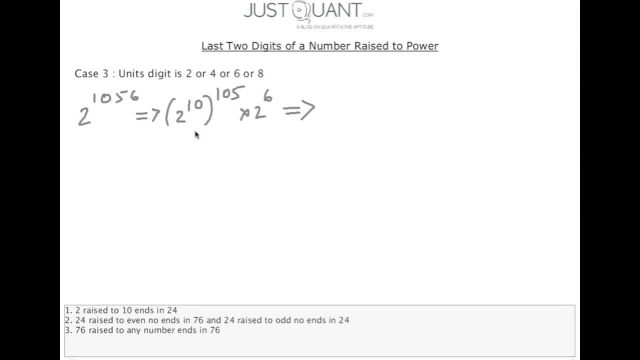 So 2 to the power of 10 ends in 24, and 24 to the power of an odd ends in 24.. Hence i can write this as: 24 into 2 to the power of 6 is 64. so 24 into 64 is nothing, but this ends in 36. that's it. so 24 into 64 ends in 36. therefore, 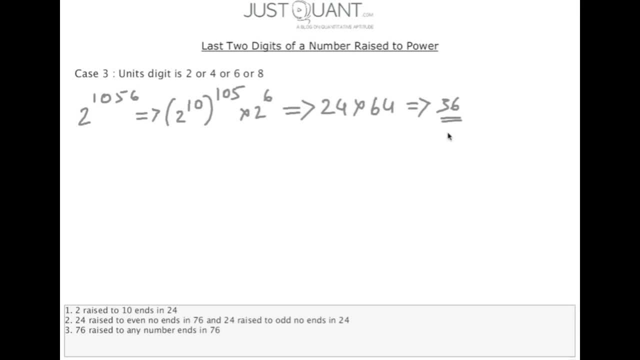 2 to the power 1056 ends in 36.. let's have a look at another example. say 84 to the power of 150.. this i can write as 21 to the power of 150 into 4 to the power of 150. 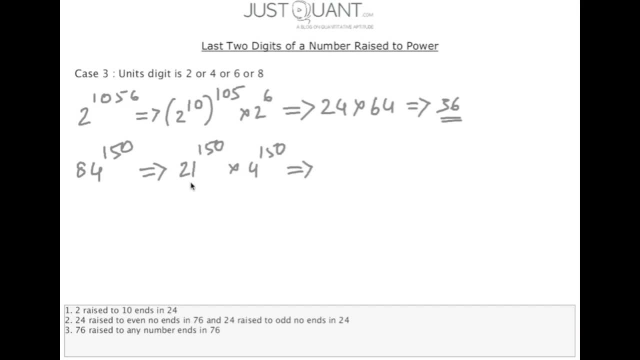 so which is equal to this is equivalent to case one wherein the units digit ends in one. so, based on case one, in the last two digits of 21 to the power of 150 is 0, 1 and 4 to the power of 150. i can write this as 2 to the power of 300. 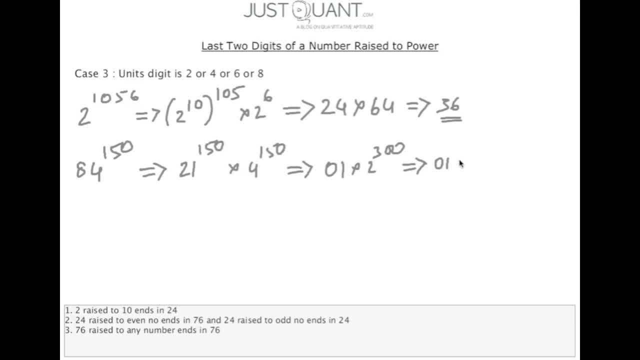 this is nothing but 0, 1 into 2 to the power of 10, whole to the power of 30, which is equivalent to 0, 1 into 2 to the power of 10, is this ends in 24 and 24 to the power of 30. 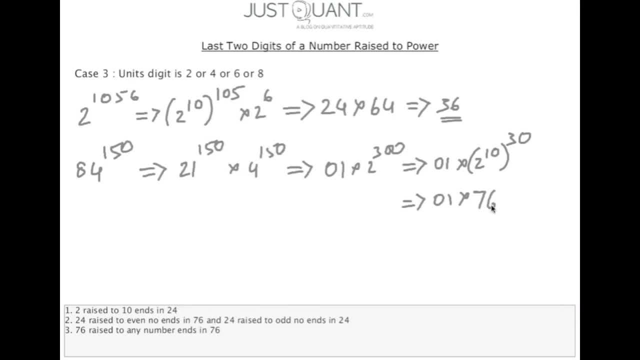 which is an even, ends in 76. so this is equal to 76. so 0, 1 into 76 will end in 76. so similarly, if you have a number, say 152 to the power of x, I can write this as 19 to the power of x into 8 to the power of x. 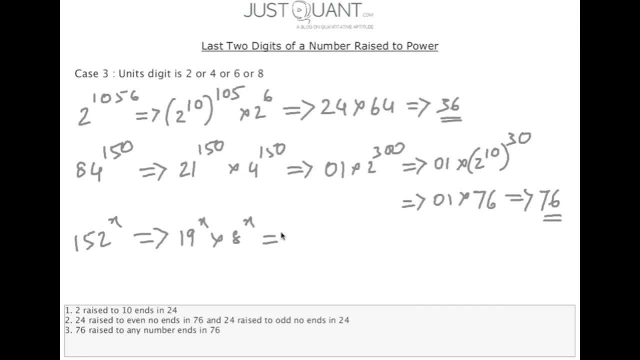 which is equivalent to 19 to the power of x, into 2 to the power of 3x, and the last two digits of 19 to the power of x can be obtained by case 2 and 2 to the power of 3. x can be solved based on how we have calculated the number of digits in this case. 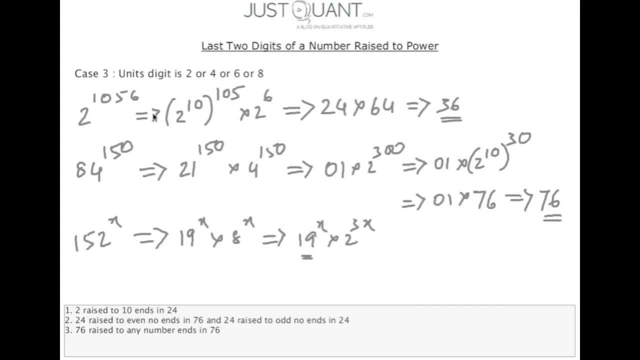 so we are left with 4 to the power of 10, based on how we have solved 2 to the power of 1056.. Once we get the last two digits of both the multipliers, we can then multiply both the last two digits to obtain the last. 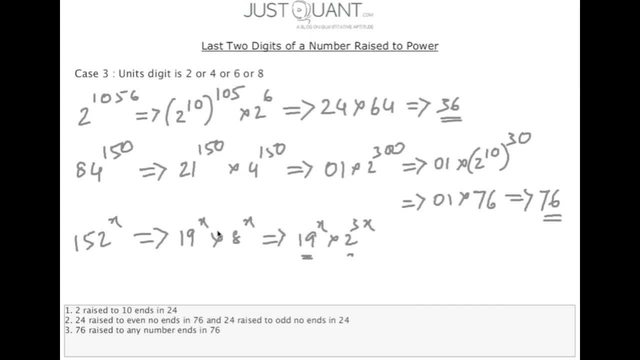 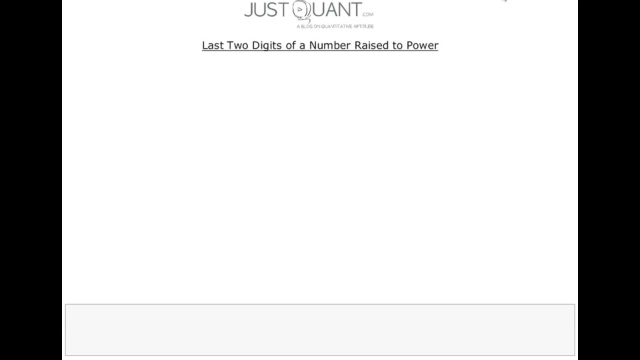 two digits of 152 to the power of x. I hope this is clear. We will move on to the next case, when the units digit ends in 5. Case 4, when the units digit is 5. Here I will use O to represent an odd digit and E to represent 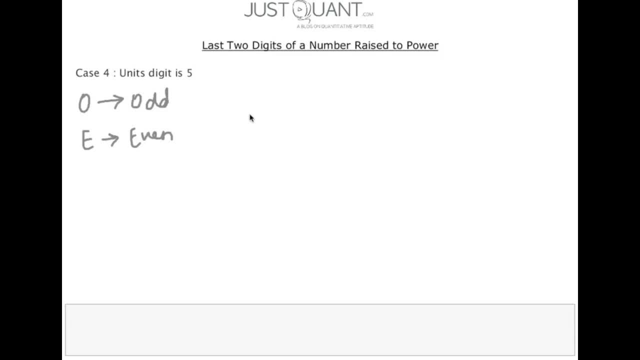 5.. So if the base ends in 5 and the digits previous to 5 is odd and the exponent is odd, then this particular number ends in 75. And if the exponent is even with the digits previous to 5 being odd, then this will end in 25.. 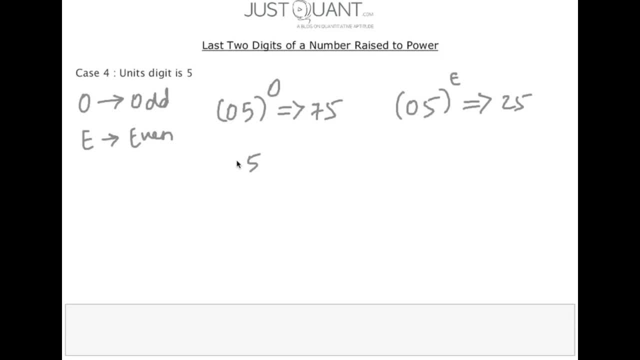 So digit previous to 5 is even and the exponent is odd, this will end in 25 as well. and if the digit previous to 5 is even and the exponent is also even and this also ends in 25.. okay, in general, when the exponent and the digit in the tens place of the base are both odd, 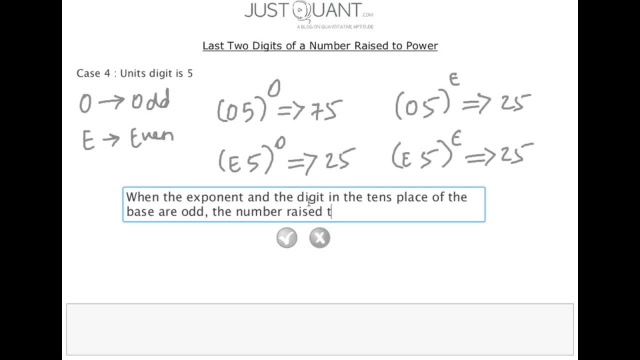 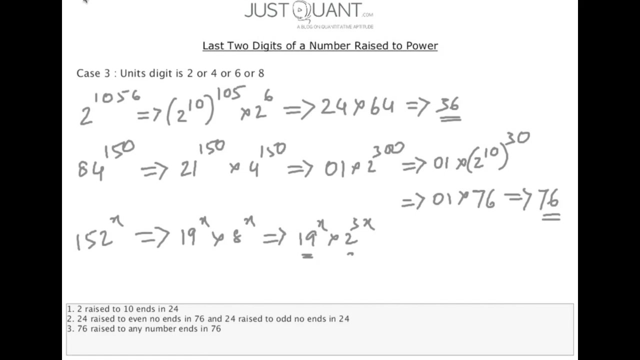 the number raised to a power ends in 75. in all of the cases it ends in 25.. so this ends our case 4.. i hope each of these cases involving the calculation of last two digits of a number raised to a power is clear. you can. 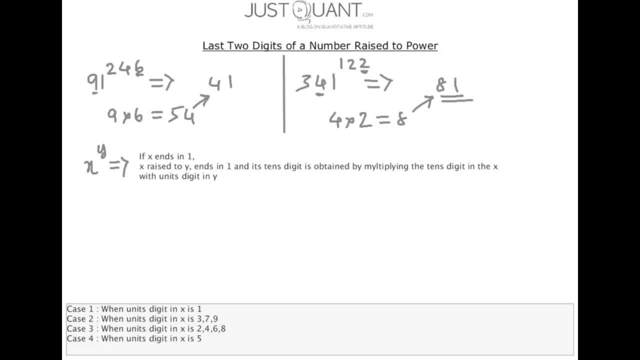 post your comments in our website, justquantcom. thanks a lot.